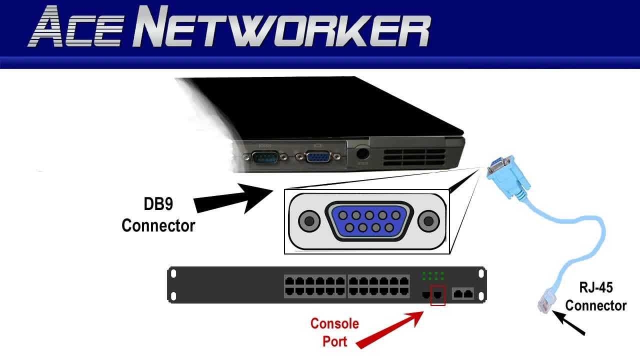 device itself, It actually can be one of the most secure, if not the most secure, access method available. So I just wanted to point that out. If you can control physical access to the device and you don't allow connectivity to it remotely- which we're going to talk about shortly- then you have really the most. 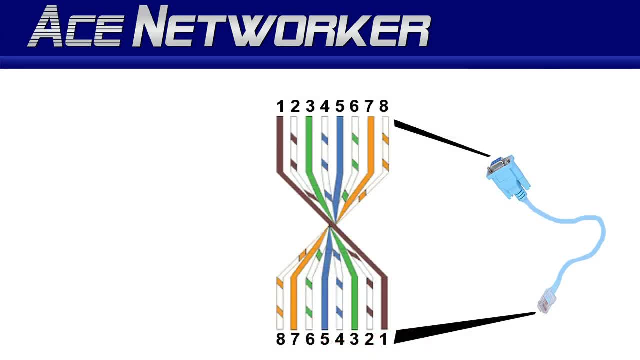 security that you can devise for that device. Now, a rollover cable is simply a cable that rolls over or maps pin 1 to pin 8,, pin 2 to pin 7, and so on, and so on. It essentially rolls over from one end. 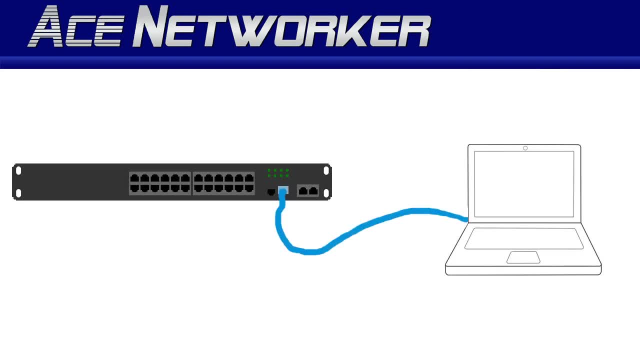 of the cable to the other end of the cable, and then it rolls over from one end of the cable to the other end of the cable to the other. That's why they call it a rollover cable. Now, once this physical connection is made, the administrator- which again may be you- uses a terminal, emulator or terminal. 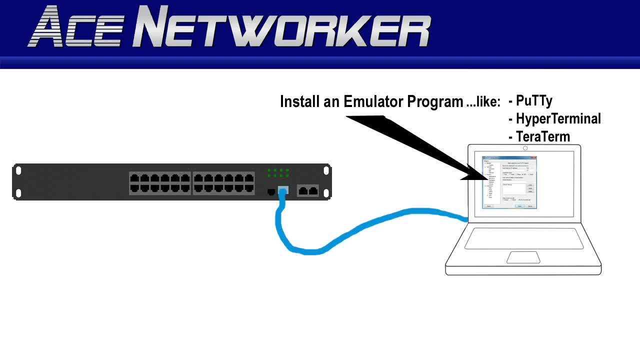 emulation program such as HyperTerminal or TerraTerm or PuTTY P-U-T-T-Y to actually type in the configuration changes using command line interface. Now, by the way, many of these terminal emulation or emulator programs can be found and downloaded for free online. All you have to do is search for. 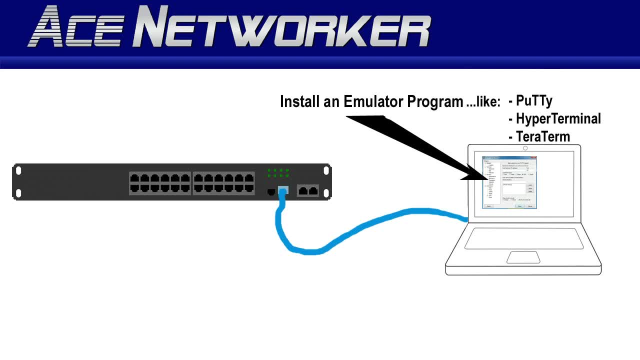 PuTTY Download or HyperTerminal download or TerraTerm download, and you can find these. There are lots of others that you can use as well. Those are the most commonly used, and you'll find multiple places for downloading those just by doing a Google search or a Bing search online. Now, once, 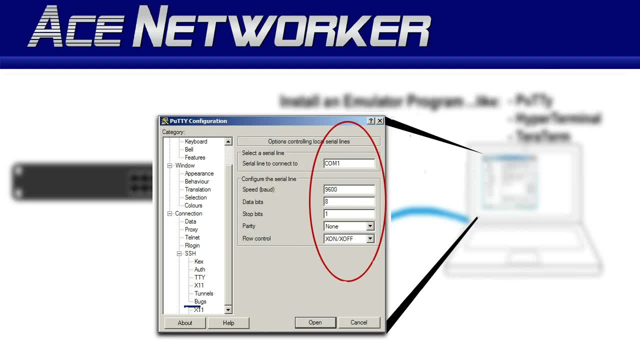 you've installed this emulator program, whatever you choose to use, to the laptop or the PC that you'll be using to directly connect to the router or the switch, the emulator program will need to be configured itself properly with the proper settings for the computer's serial port to allow. 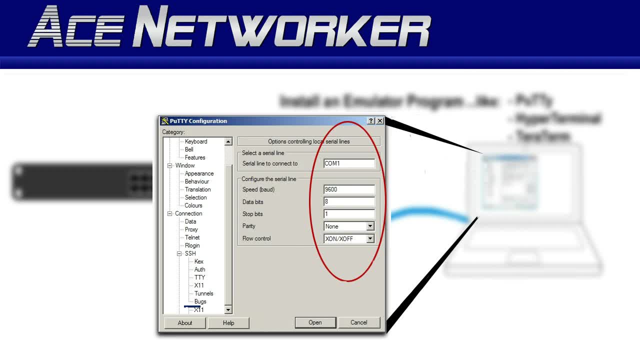 that switch or the emulator to be connected to the router or the switch. Now, once you've installed that switch or that router's settings to display in the program window and to accept your commands, the default setting for most industry switches and routers is as follows. It's usually 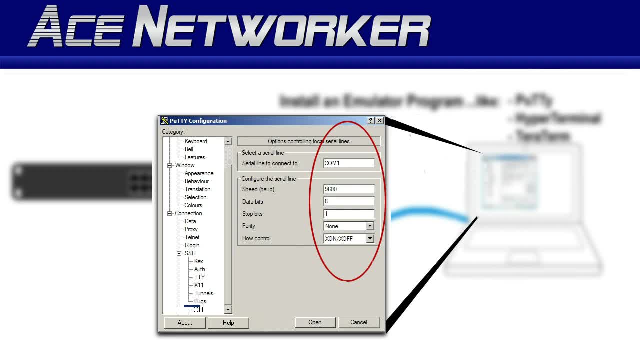 9,600 bits per second. on the speed, I have seen some switches and routers, some brands with higher speeds and I in fact I saw one with a slightly lower speed, but it typically the industry standard is 9,600 bits per second. You will never have any hardware or flow control or flow control. 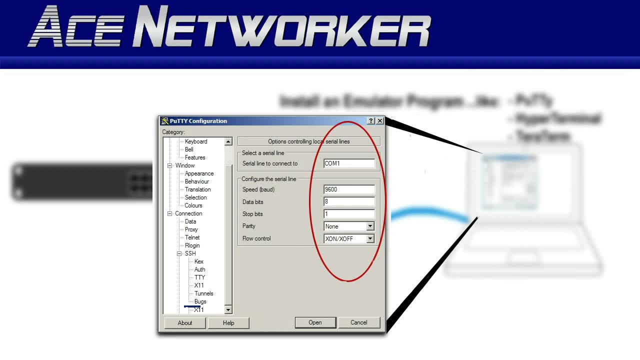 is disabled, It's going to be eight bits- ASCII setting and the stop bit is going to be eight bits. The stop bits are always set to no, no stop bits, and parity bit is always set to one. Once the communication settings are in place, the emulator allows access to the device and usually you can. 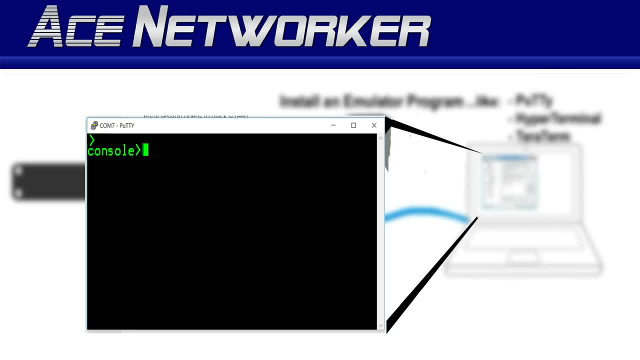 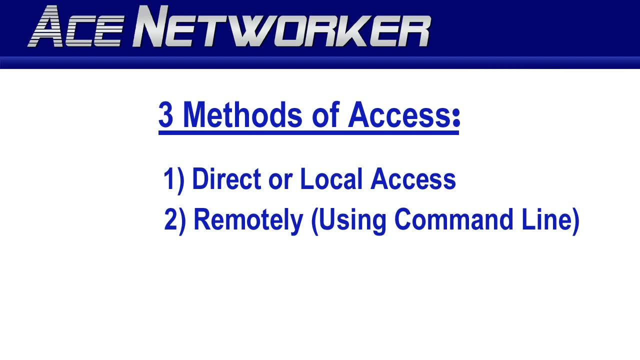 test this by simply tapping the Enter key to see if you get a console prompt on the screen or in that window for that emulator. Now an administrator- and this again may be- you can also access a network device remotely using command line interface. Now this is done through two methods. 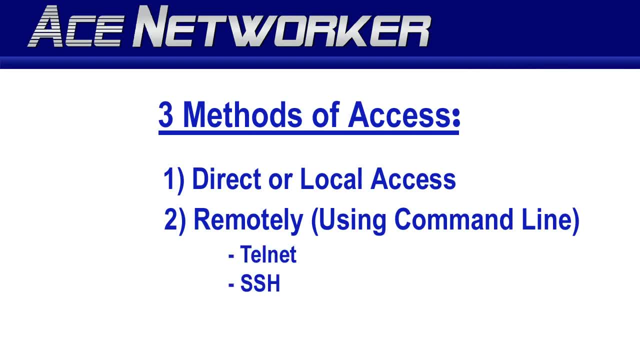 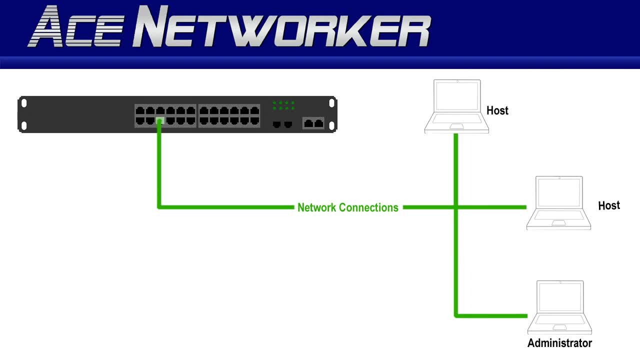 You can do it through Telnet or you can do it through what they call SSN. Now, the SSN is a SSH. A Telnet or SSH session between the administrator's PC and the router or the switch provides the same functionality as a direct console connection that we just discussed. 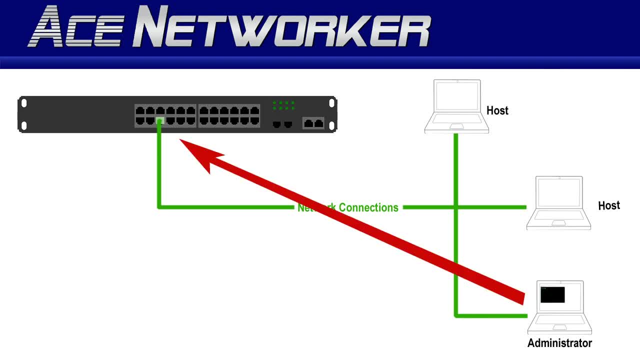 The benefit of this is that the administrator can access configuration files on a switch or router without having local direct physical access to that switch or router, And they can do this from any location inside or outside the network. So if they're several hundred miles away, or a couple, 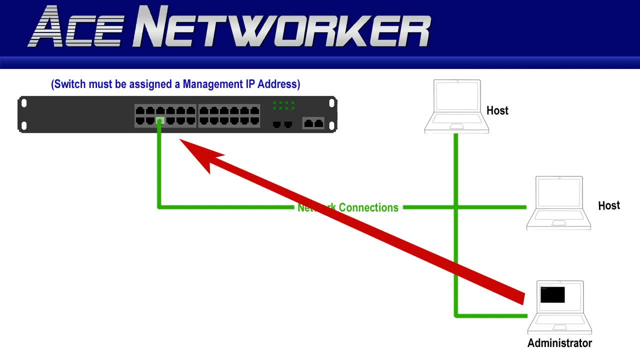 thousand miles away. it doesn't matter. They can be on the other side of the planet, but if they have access to the network, they can usually access these settings using Telnet or SSH. The drawback to this method, obviously, is the security that you run into, the security. 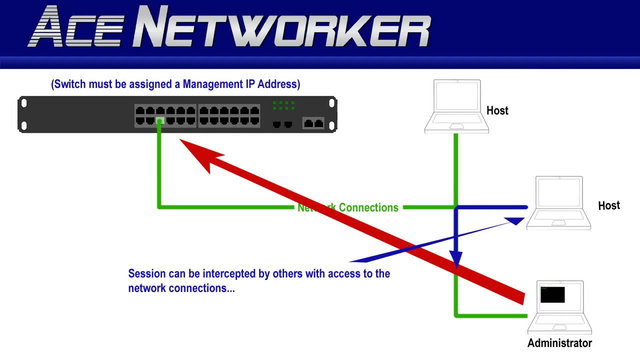 risk that you run into, Because allowing remote access through any method opens a security concern on your network. Now, if remote access to devices is a necessity, the device must be configured to allow this access. You actually have to set this up on the switch or router for. 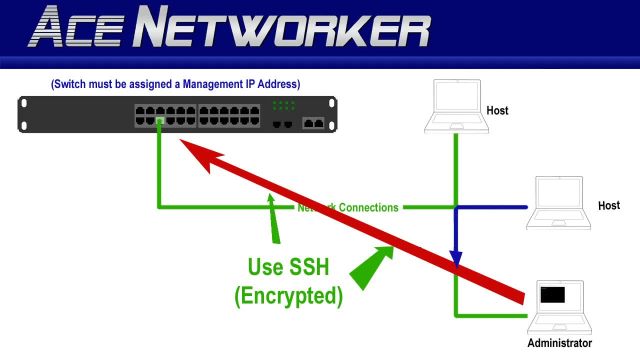 it to work. SSH should be used- and it's always recommended- in place of Telnet, Because SSH uses an encryption that, even if detected or if somebody picks up that connection and they're able to read off of it or see it, it's still encrypted, So it doesn't make any sense to them. 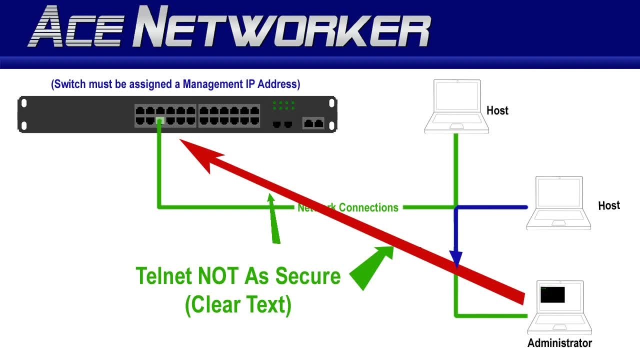 However, via Telnet there is no encryption. So if someone picks up that connection between the administrator or you connecting to that from wherever they are across a network, to the router or the switch, they're not going to be able to access that connection. So if someone picks up